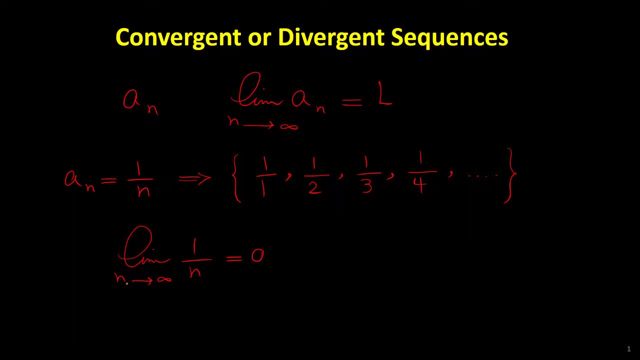 infinity, 1 over n approaches 0.. So this sequence is convergent and converges to 0.. Let's do another example. So we have 1 over n plus 1.. First term of this sequence is 1 over 2.. The second term of this sequence is 2 over 3.. 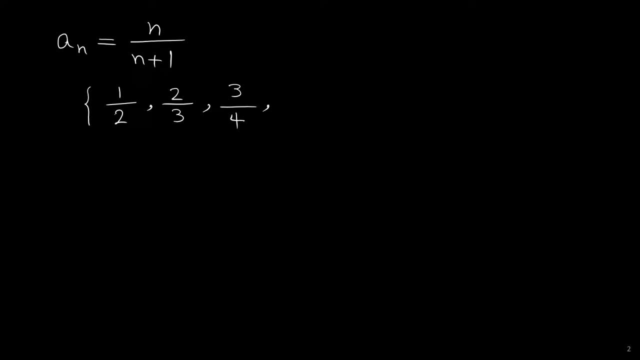 The third term of this sequence is 3 over 4.. The fourth term is 4 over 5, and so on. It seems that this sequence is also convergent. But what is the limit of this sequence? To find the limit of this sequence, we have to find limit of n over n, plus 1 as n approaches infinity. 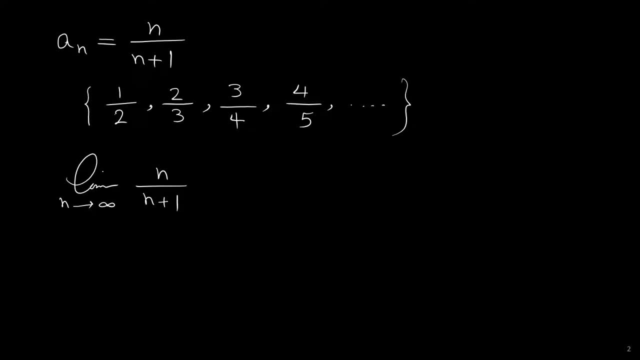 We know that when n approaches infinity, to find a limit we can consider the dominant terms of the top and the bottom In this limit. the dominant term in the top is n and the dominant term in the bottom is also n And we can ignore this 1, because 1 compared to n is nothing, and we can ignore 1 in the denominator. 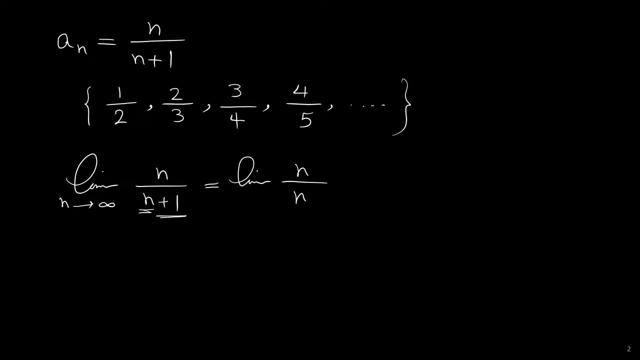 Note that n approaches infinity and 1, compared to infinity, is nothing, and so we can eliminate 1 in the denominator. If we do so, limit of n over n, as n approaches infinity, equals 1.. Another way that we can find this limit is to find the dominant term in the denominator. 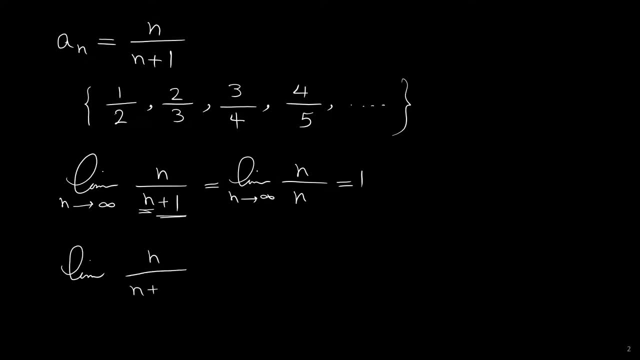 is to divide top and the bottom of this fraction by the highest degree of denominator. if we divide top and the bottom of this fraction by n, we have n over n over n over n, plus 1 over n, n over n. in the numerator is 1, n over n. here is also 1, and we know that 1 over n because n approaches infinity. 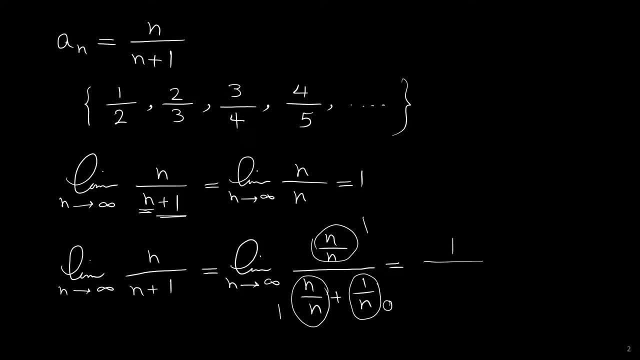 is 0, so we have 1 over 1 plus 0, which equals 1. we get the same result as the previous method. so limit of this sequence is 1, and so it shows that the sequence is convergent. another example: consider this sequence: a n equals 2 negative 1 to the power of n, first term of this sequence. 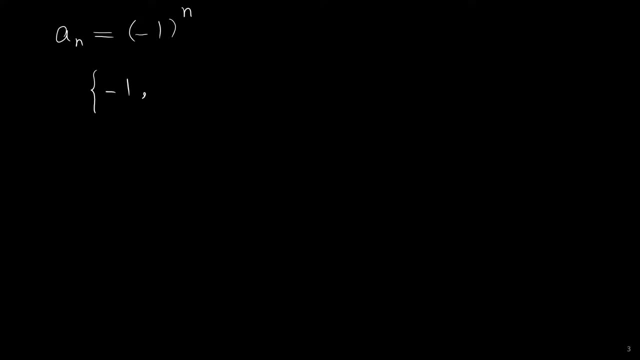 is negative 1, because negative 1 to the power of 1 is negative 1. the second term is negative 1 to the power of 2, which is 1. the third term is negative 1 again. the fourth term is 1, and so on. 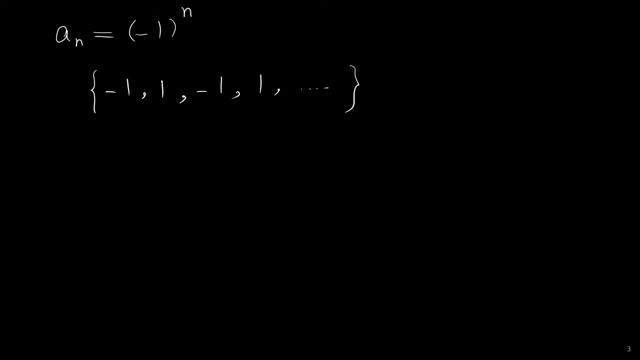 you, because the terms of this sequence alternating between negative 1 and 1, this sequence is divergent and never the sequence approaches a single value. so we say sequence a- n is divergent because it doesn't approach a single value. now look at this example: n to the n over n- factorial. 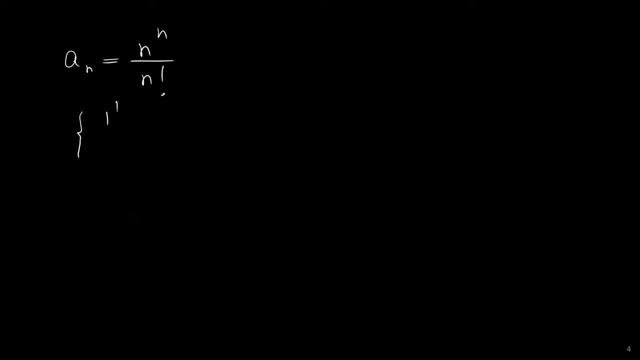 the first term of this sequence is 1 to the power of 1 over 1 factorial. the second term is 2 to the 2 over 2 factorial. the third term is 3 to the 3 over 3 factorial. the fourth term is 4 to the 4 over 4. 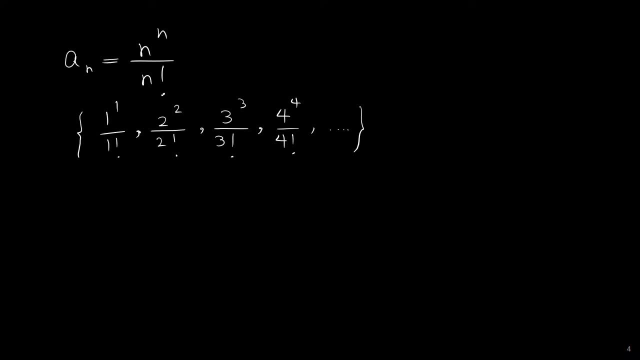 factorial and so on. if we simplify these fractions, 1 to the 1 is 1, 1 factorial is 1, so the first term is 1, the second term is 4 over 2, factorial is 2, 4 over 2 is 2.. the third term is 3 to the 3 is 27 and 3. 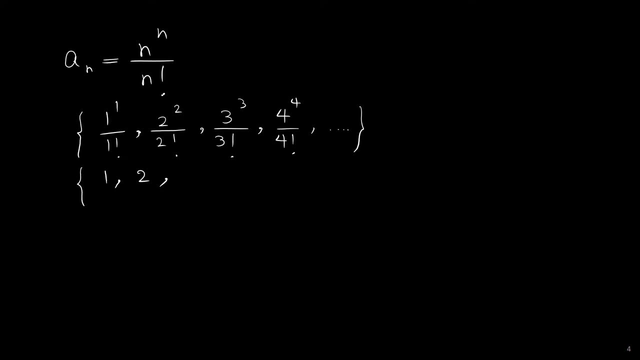 factorial in denominator is 6, 27 over 6, which can be simplified to 9 over 2.. 4 to the 4 is 256.. and 4 factorial is 24.. if we simplify top and the bottom, we can write 256 over 24, as 32 over 3. 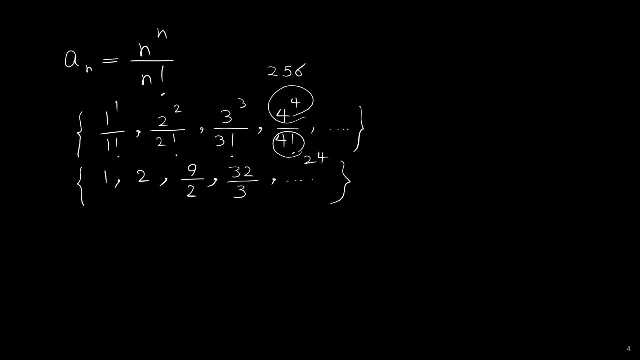 by looking at the values of the terms of this sequence, we can see that the magnitude of the terms increases without Bond. the first is 1, the second term is 2. the third term is 9 over 2, which is 4.5. the fourth term is 32 over 3. 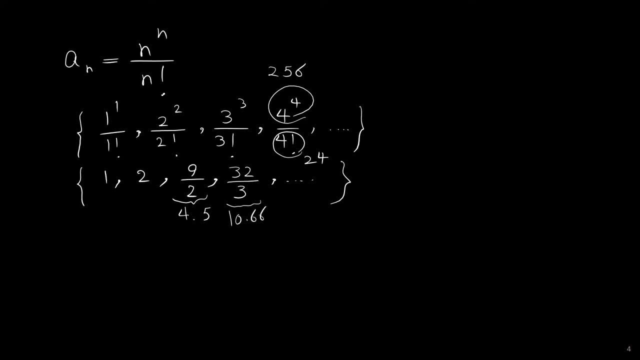 which is 10.66, and so on. as you can see, the values of the terms increases without any bond and if we continue writing the terms, they become larger and larger. so the sequence diverges. but how we can prove that this sequence diverges? we want to find limit of n approaches infinity n to the n. 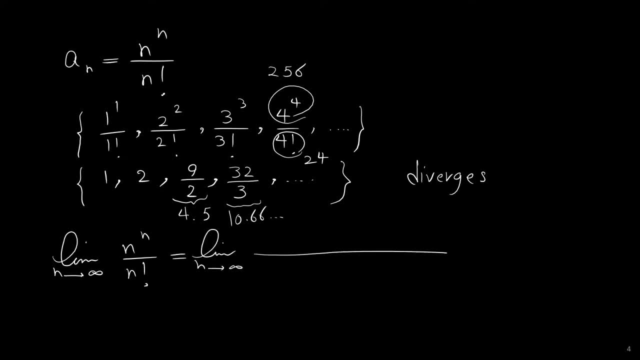 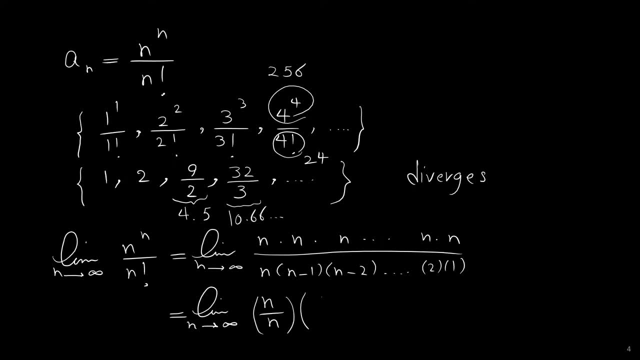 n over n times n over n. minus 1 times n over n, minus 2 times n over 2 times n over 1. as n approaches infinity, n over n is 1.. The value of the second fraction is also greater than 1. value of the third fraction is also.